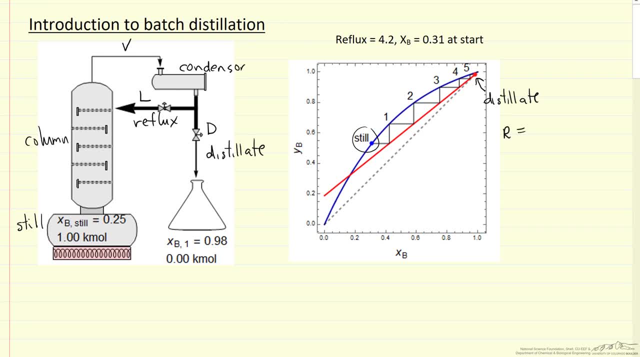 and the reflux ratio is the liquid flow rate over the distillate flow rate And then the slope of this line is related to this reflux ratio and this is related to this reflux ratio. So batch stills are used typically if we have smaller quantities that we want to separate. 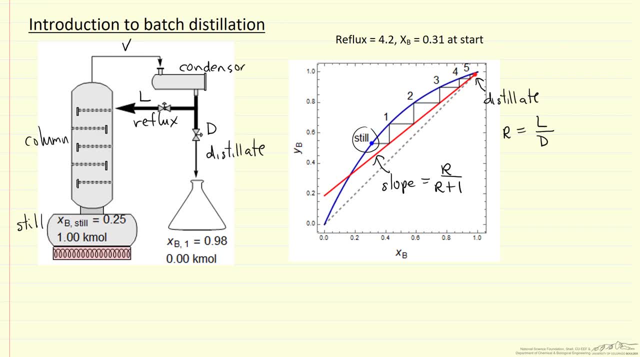 They're a lot more flexible. The same system can be used in sequence for different mixtures. It also allows each batch to be identified. You know what would exact feed conditions be, conditions where we carried out how long, etc. And for pharmaceuticals or for food, this could be important. 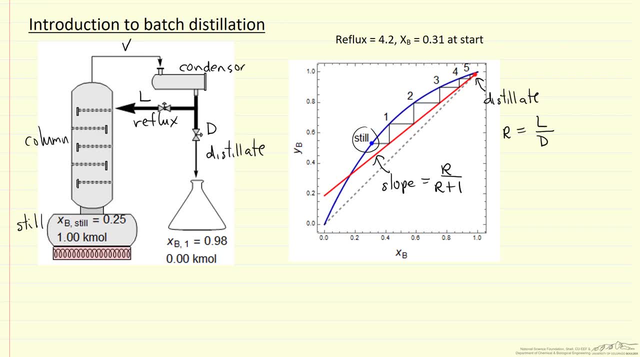 So, So So. the typical way that this would be run is we start out, where we close this valve and we completely reflux at the start and let the system get to equilibrium. This allows us to get the best separation. Then we open the valve and start collecting. 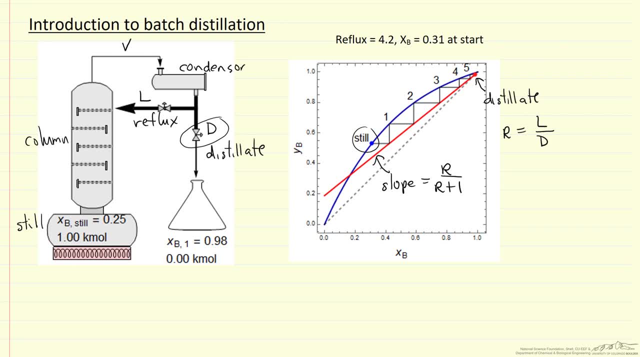 Now, unlike the diagrams you see, say for continuous distillation, the McCabe-Thiele type diagrams, as we distill the liquid, the mole fractions in the still change, and the mole fraction of the distillate change, which means this red and the blue points are moving, which means the line is moving, the red line is moving. 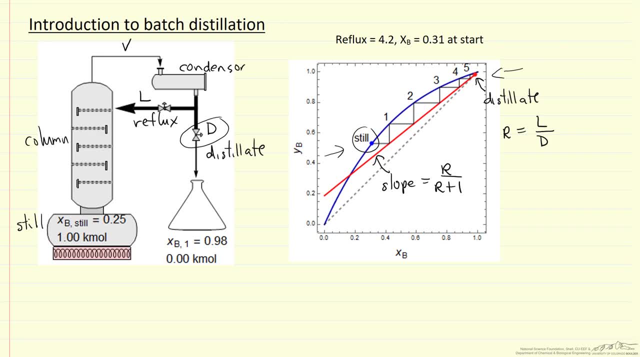 The blue line is just equilibrium data, so that doesn't change. But the red line is going to move as distillation proceeds, but the slope remains the same: just r over r plus 1.. So let's look at what this y-x diagram would look like at a later time. 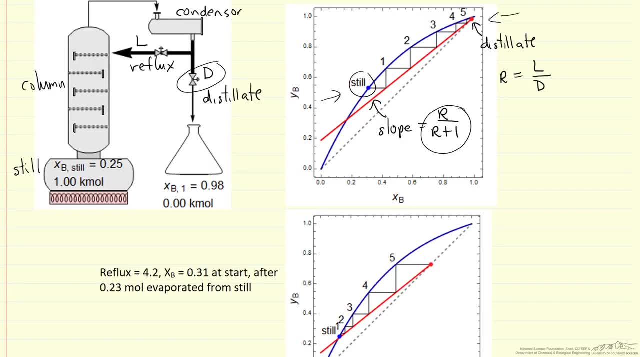 So here I'm showing the same y versus x figure. but now we've evaporated 0.23 moles from the still. So that means, the distillate composition has changed significantly and the still composition has changed. so the diagram, the operating line moved. 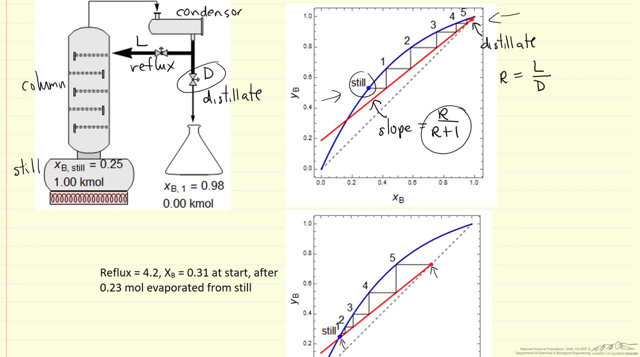 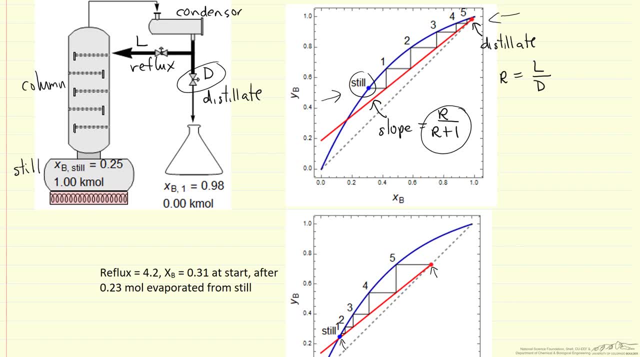 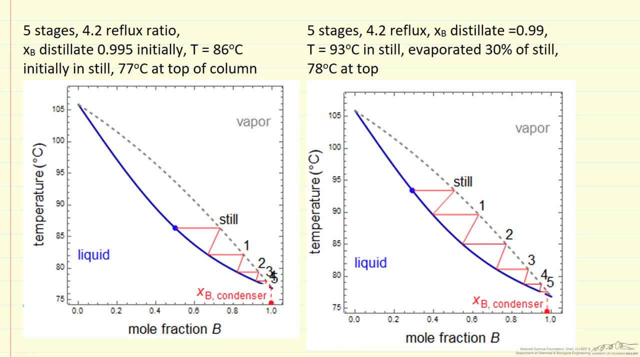 Again, the blue line corresponds to vapor-liquid equilibrium, and the stages are counted off by referring to the y-x diagram in the operating line. there, The point that's important here is the- this is the case- five stages and the temperature. 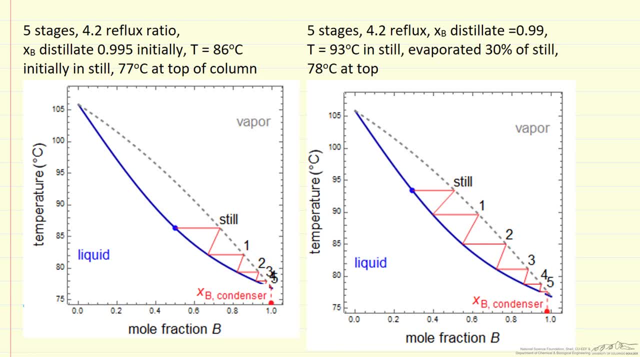 is 86 degrees in the still when we start, but it's only 77 degrees at the top of the column. so 86 degrees- you can see the blue and then 77, it's a little harder to see this red point here. 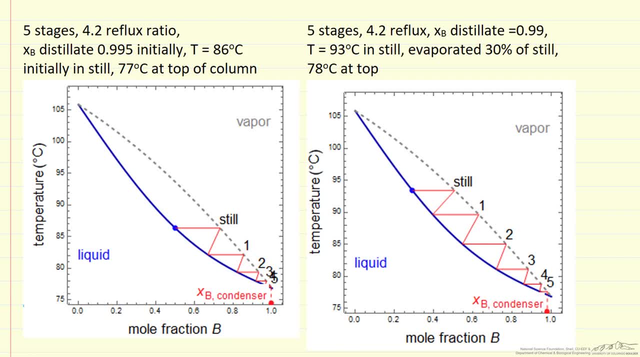 And then, after we've evaporated 30%, notice the stages. the locations have changed. the temperature's now 93 degrees in the still and then 78 at the top of the column. Look at one more figure where we've evaporated even more.